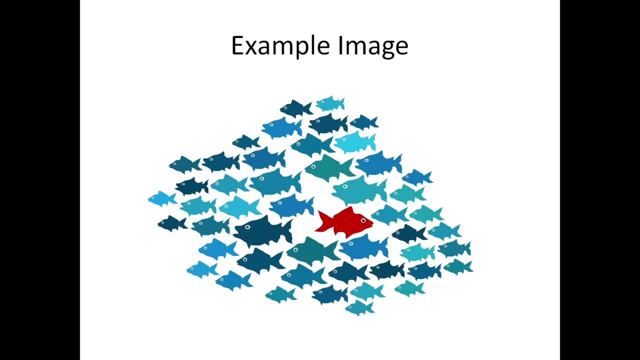 dataset For identifying the anomalies. we need to create a program which will detect the anomalies that are present in the dataset. Detecting the anomalies is very different for different datasets. If you have less noise in the dataset then you can find the anomalies easily, But if 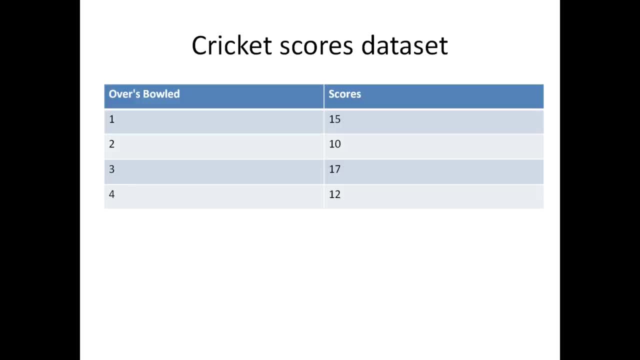 you have high noise, it is a very hard process for detecting the anomalies In this video. I am going to explain with the crickets course dataset. I just modified the dataset for this video. This will give you the clear-cut explanations of anomalies. 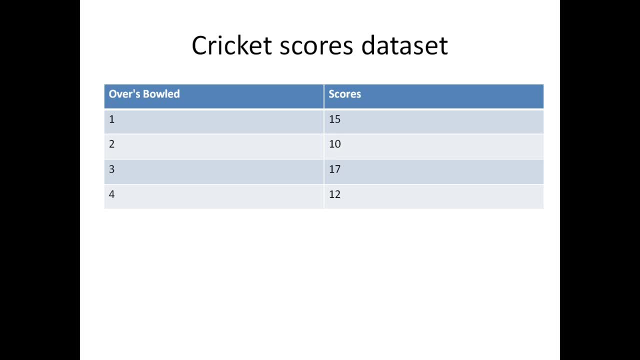 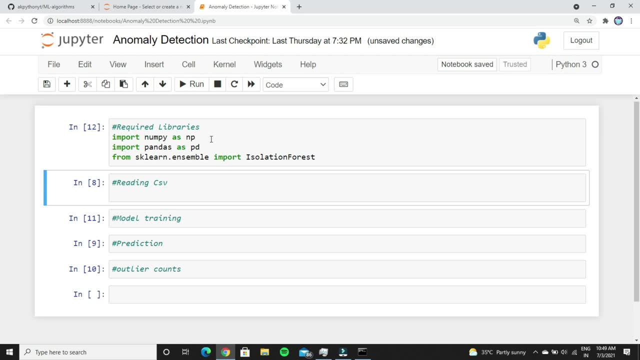 detection concept. So watch this video fully to understand the entire concept. Here I imported the required libraries for this problem. Let me give the library explanations. NumPy is for performing the array operations. Panda is for real-world data collection. Finally, from the sqln library we imported the isolation forest module. That is very 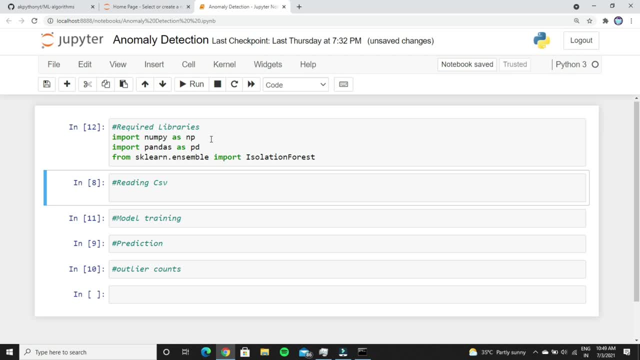 important for this problem. So the isolation forest is used to create a tree-like structure based on the data points we have. It builds the tree-like structure based on the closest relationship between the root value and the child value. This module will form the trees. 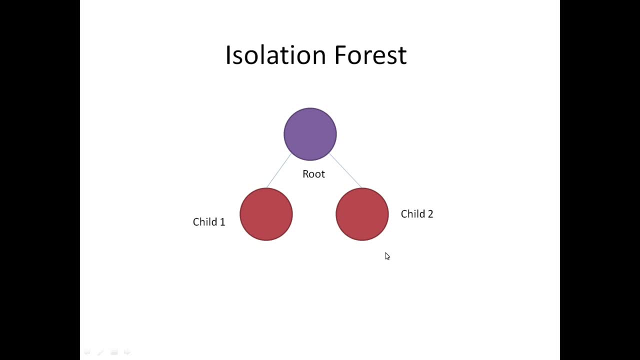 according to their closest relation. In the isolation forest you can decide how many tree values we need to form. Forming a tree is an iterative process in this library. If you want to perform 50 iterations, then you will get some kind of accuracy, Accuracies. 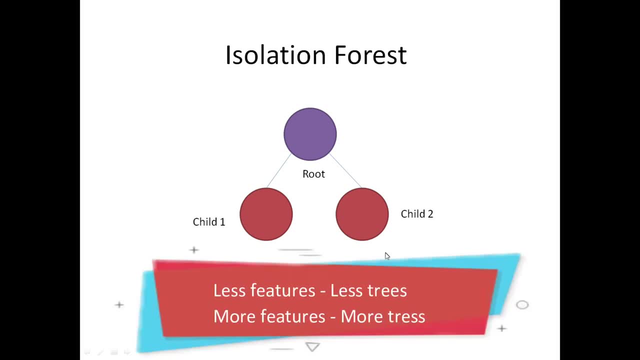 based on the data you have. Okay, Suppose, if you have less features of data, then the less amount of tree formation is enough to process the data, And if you have large features of data, then you need to form nearly a hundred trees, or more than a hundred trees is enough. 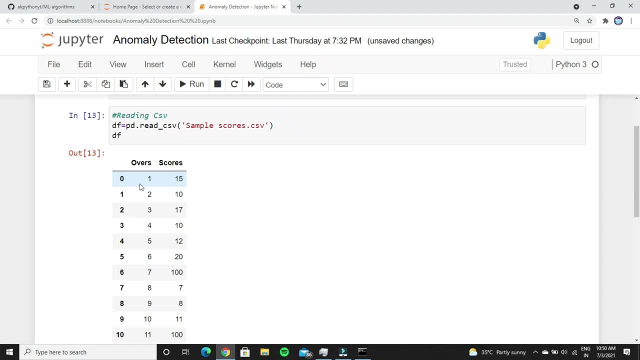 to process the data. Here I read the dataset of mine. It's a cricket score dataset which was built by me. Now look at my data values here. There are 20 ovals are present in the And in the scores column. contain the data of scores which was scored in each overs. 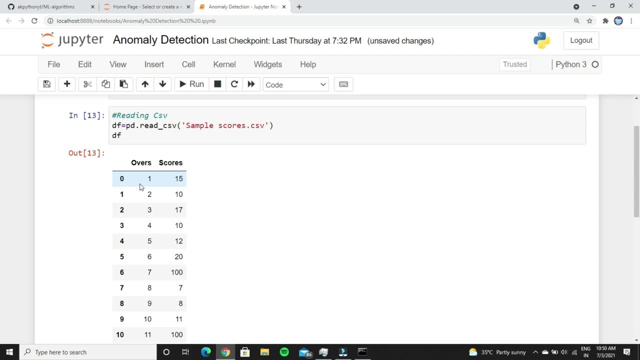 So, before we find the anomalies that present in the data set, I want to make some assumptions. In a cricket match, anything can happen, in particular overs. We can assume only 36 runs or less than 36 runs, or possible runs to score in a single. 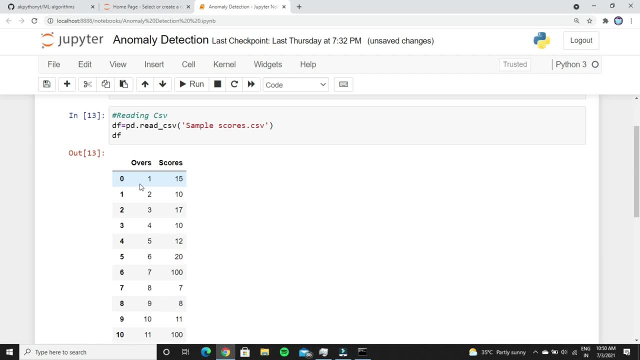 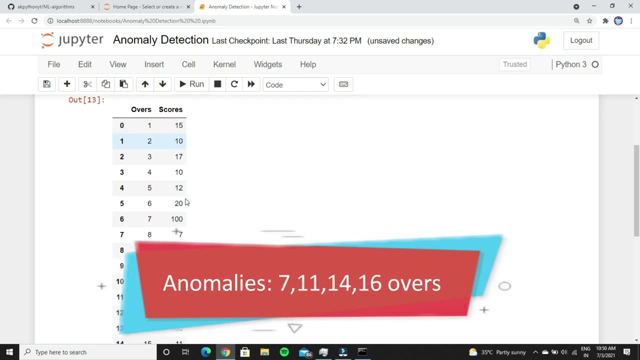 over And I made the data set like that. So look at my data set. you can simply find the anomalies by saying it in the over of 7,, 11,, 14,, 16 contains some values which are not possible to score in a single over. 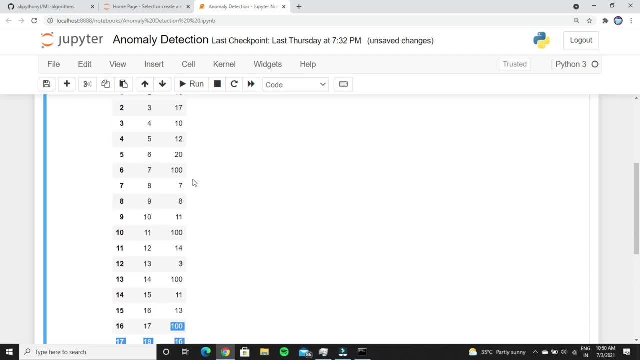 These are the anomalies that are present in my data set And it is only for explaining purposes. but in the real time you need to solve a big problem with a more complex data set. So next step, you need to create a isolation forest model, create a variable model and 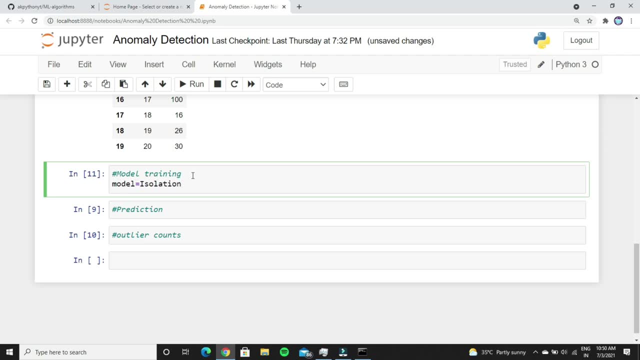 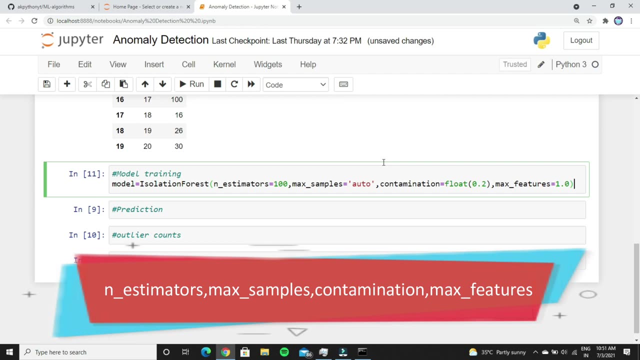 create an object- isolation forest. In this object you need to pass these four parameters. they are very, very important for tuning the model performances. Let's see its explanations. N estimator indicates how many iterative trees you need to form from these data points. 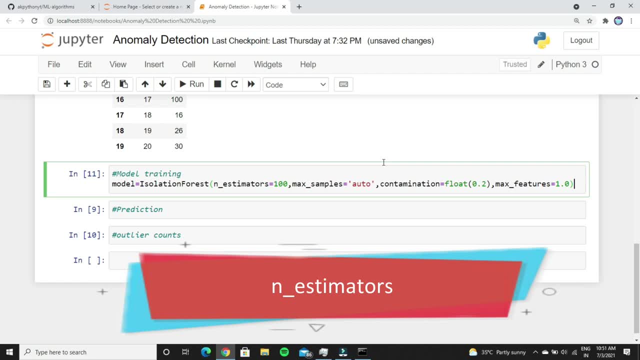 Suppose you can take the powerplay overruns when you give the N estimator value as 50, it will form 50 trees by using only the powerplay runs. I will post a decision tree algorithm video on next. You can easily understand those concepts and then you can easily relate that with this. 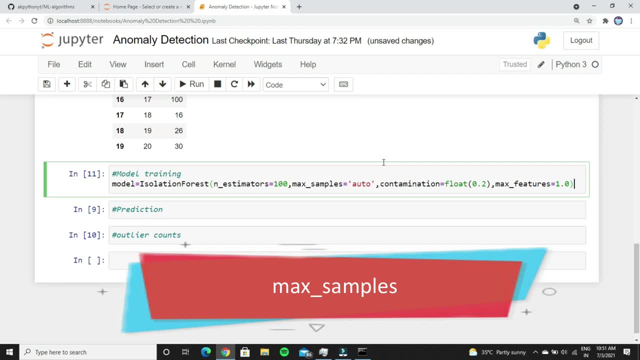 parameter. Next one is the maximum samples. Maximum samples is a kind of an allocation tool that is used for how many data samples will this algorithm take from the training data set Here? I gave the value as auto. that means I just gave a permission to this algorithm. 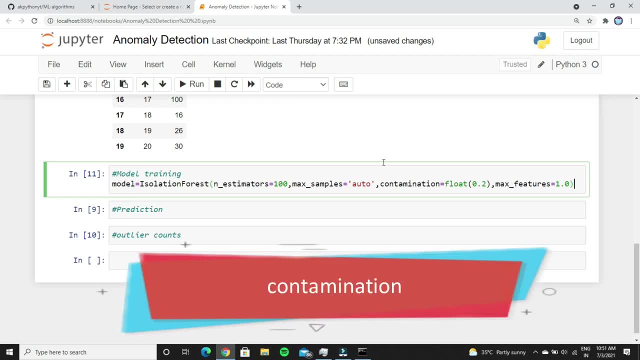 so it can take any number of samples from the data set. The third one is the contamination. Contamination means the percentage of randomness that may be present in our data set. With the help of this parameter, you can easily find out the anomalies. 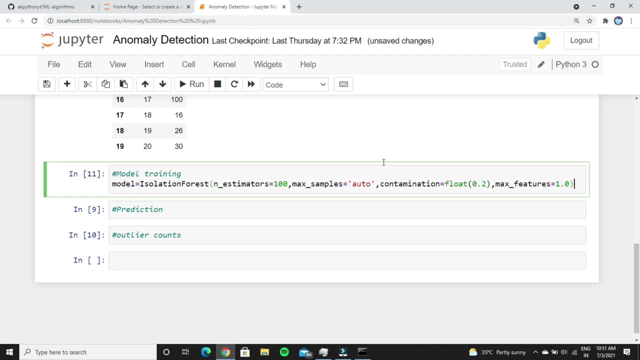 And the final one is the maximum features. It means in some data set there will be a lot of features may be present. This parameter will allow you to select how many features you need to include while training the algorithm. Here I gave the value as 1.0.. 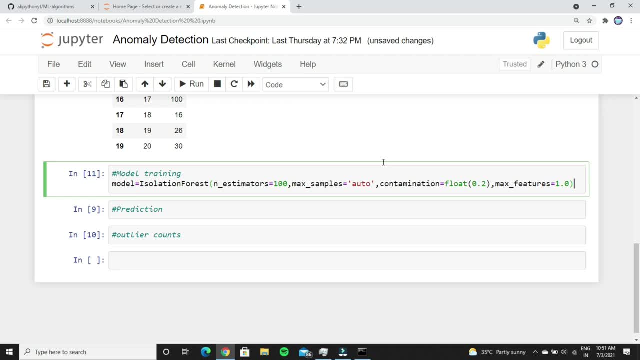 It means it draws single feature from the data set and using that feature, it will start to train the data with this algorithm. These are the important parameters you need to know in the isolation forest algorithm. I think I explained all the things And if you have any doubts about this, then comment down your thoughts.